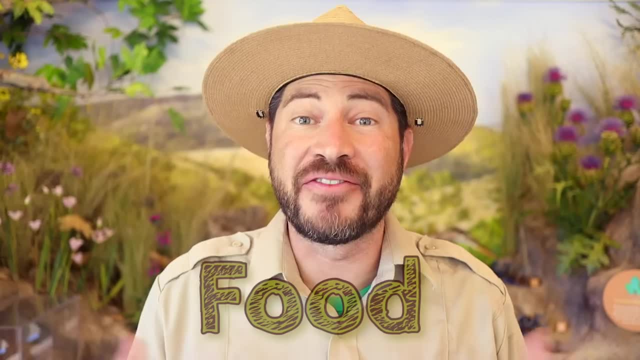 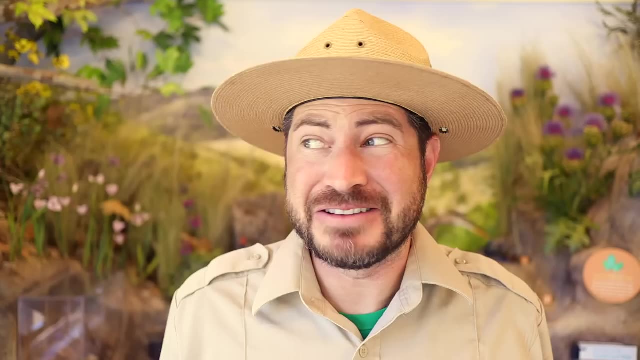 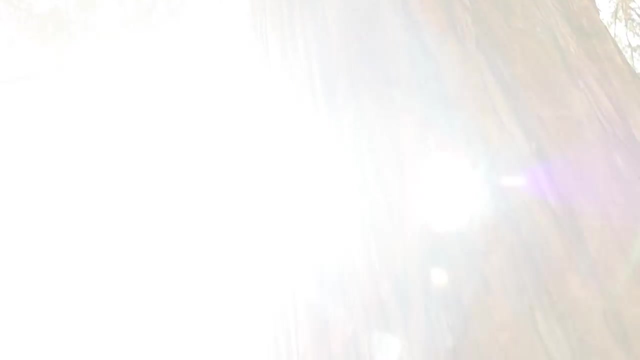 So let's think about that. at to be home, you need plenty of food for all the plants and animals that live there. some animals eat plants, some eat bugs and some eat well other animals, and this relationship creates what we call a food web. every food web starts with the sun, and this is because plants use the sun to make their 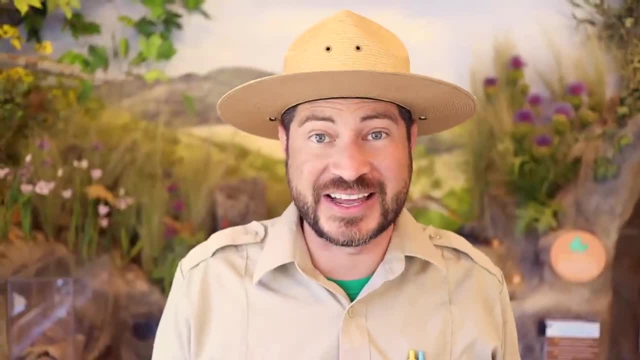 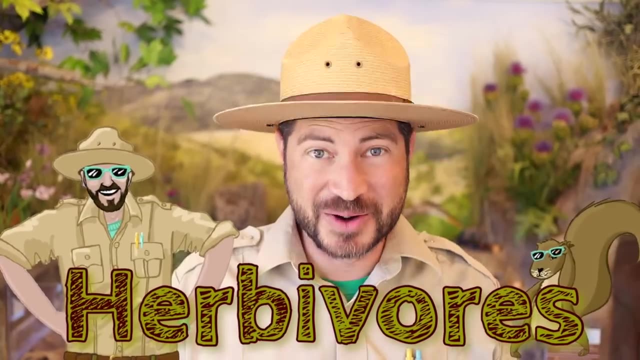 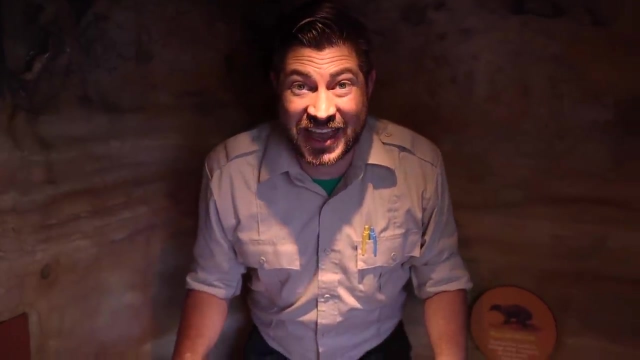 own food. now there are animals out there that only eat plants, like deer, gophers and rabbits. when an animal only eats plants, they're given a special name: herbivores. do you remember when i told you that some animals eat only meat? these animals are called carnivores. 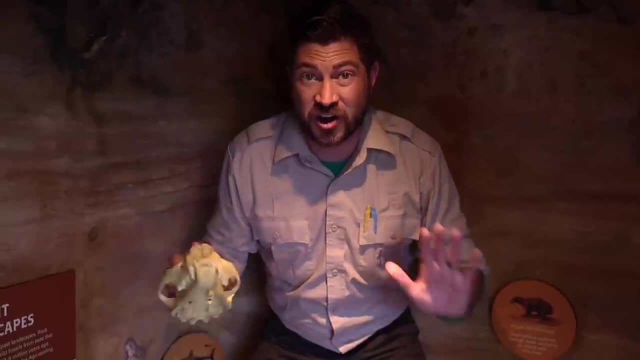 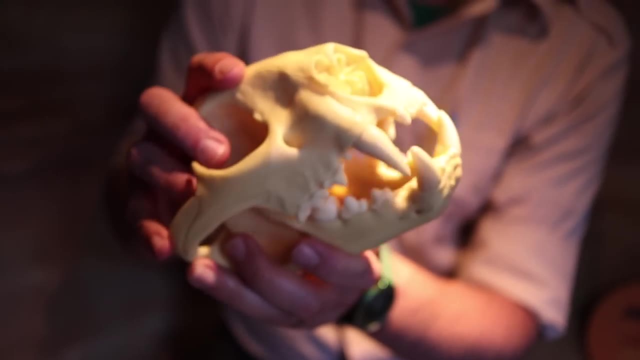 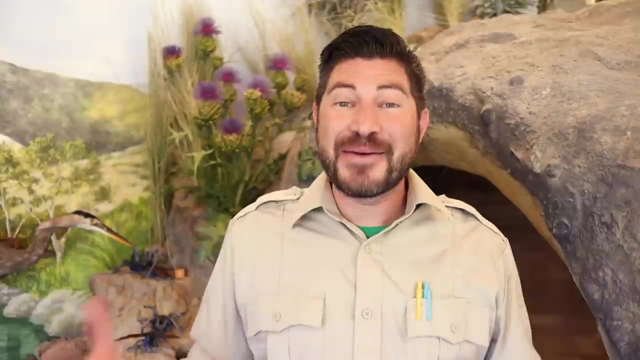 birds of prey, snakes, sharks and mountain lions are all carnivores and they eat meat. check out these teeth. these belong to a mountain lion. these sharp teeth help a mountain lion catch and eat their prey. habitats are home to animals that aren't picky eaters either. these animals eat both plants and other animals. they're called omnivores. omnivores include bears, squirrels and even coyotes too. habitats are also home to decomposers like insects, fungi and bacteria, and they feed on decaying organic matter. and they're also home to other animals like insects, fungi and bacteria, and they feed on decaying organic matter. 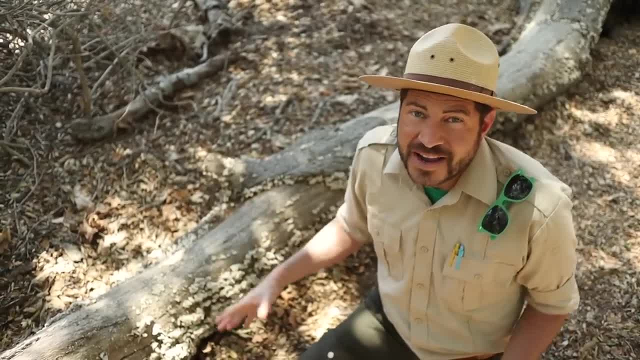 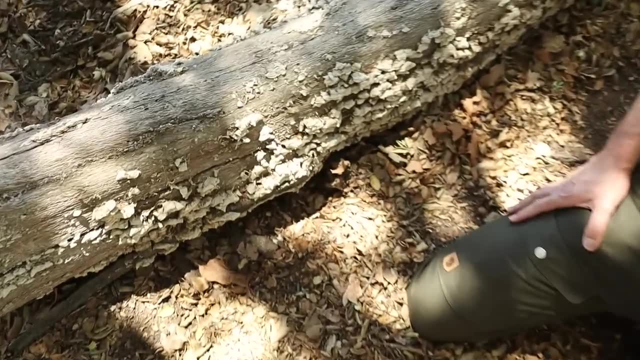 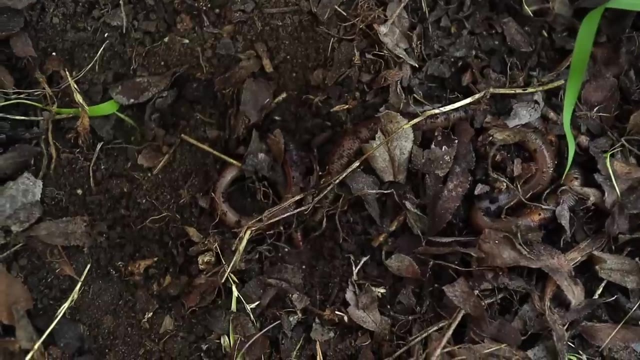 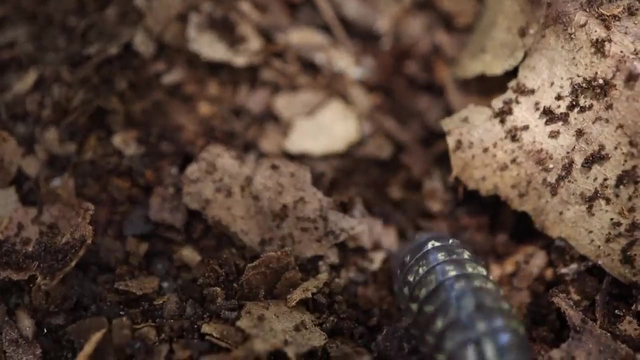 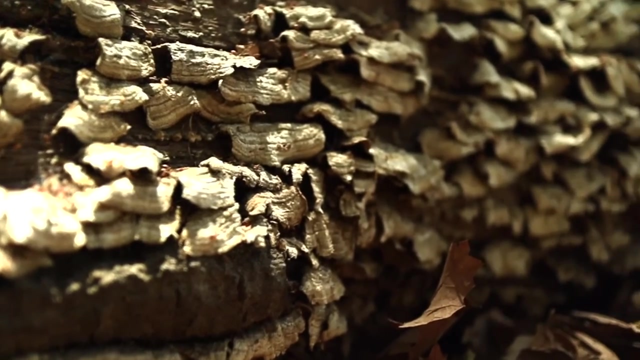 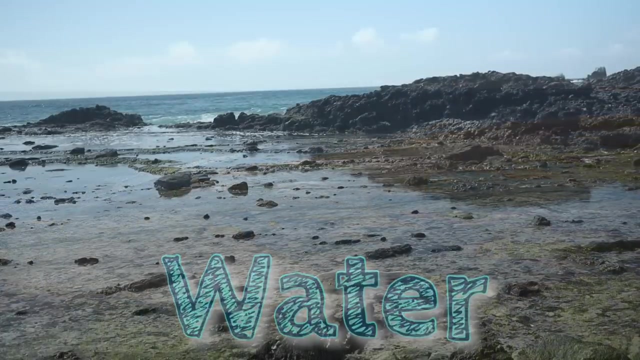 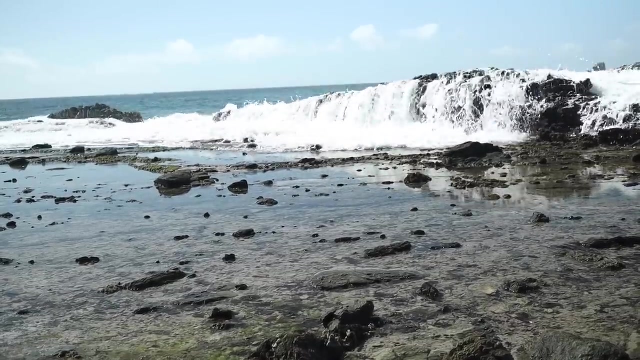 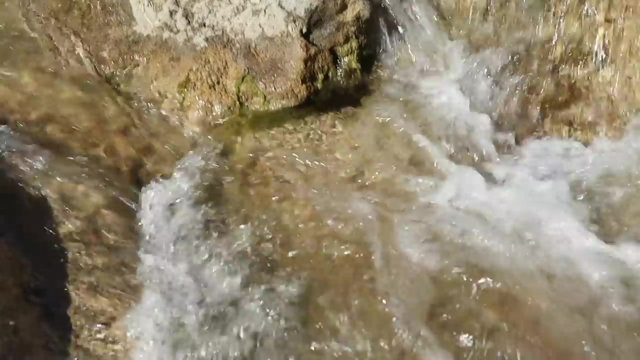 like dead plants and animals and even poop, but just look how many decomposers have made this old log their habitat. so this is what yourrisk does. the next thing that we need to make a habitat a home is water. all plants and animals need water to live, and some habitats are lucky enough to be full of it. 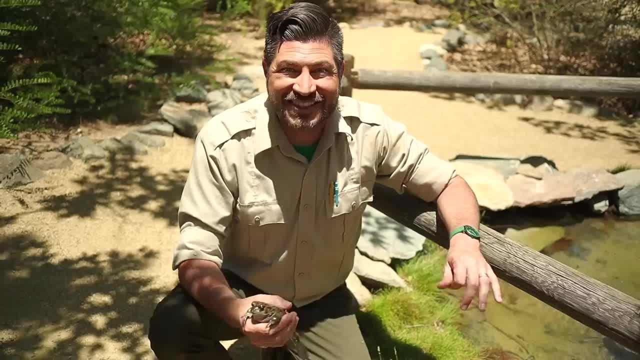 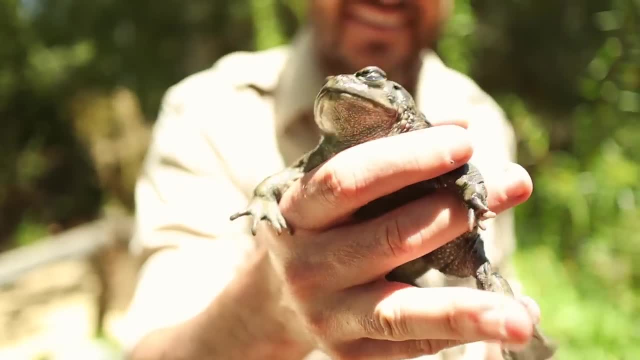 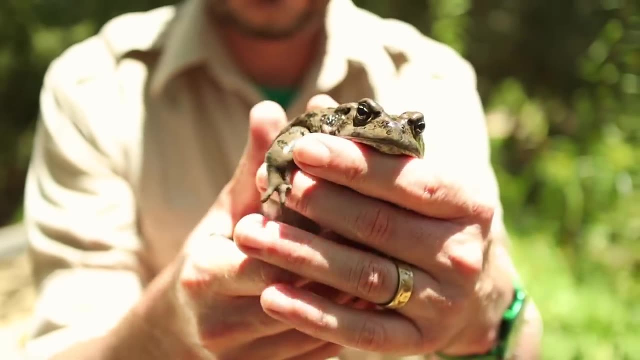 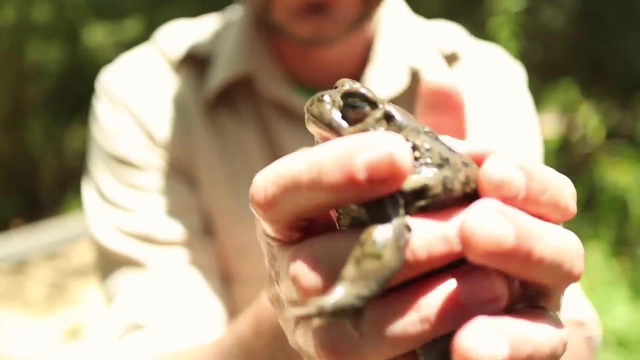 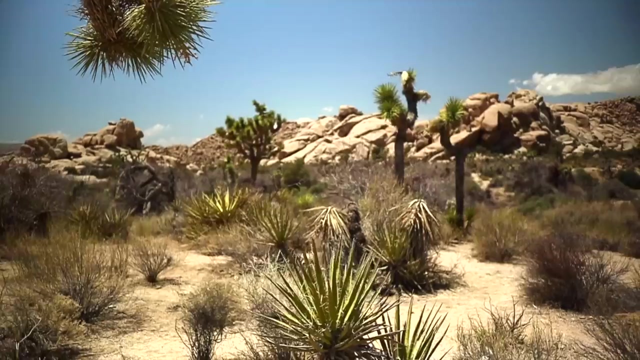 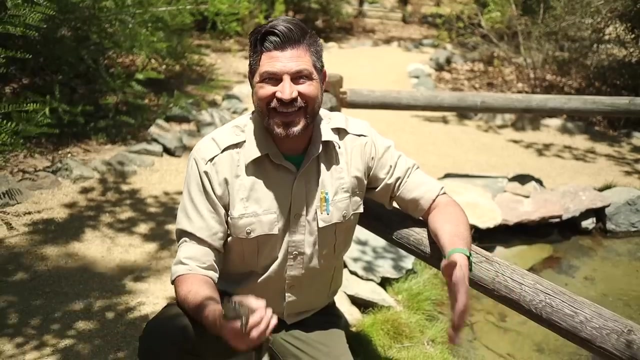 like lakes, rivers, swamps, pond, like this one where this western toad has made its home. But some habitats don't have a lot of water. Can you think of one? That's right, the desert. So the plants and animals that live in desert environments have 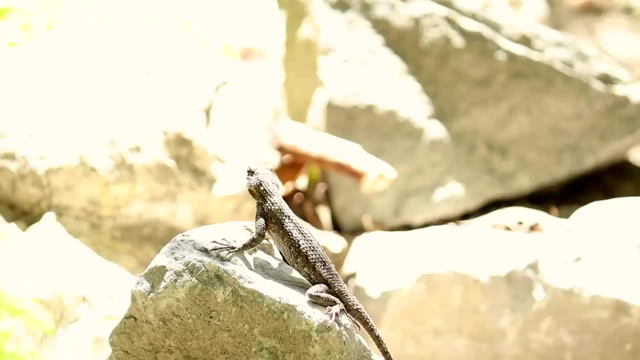 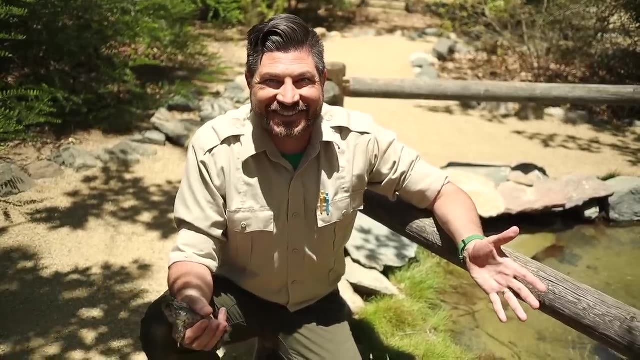 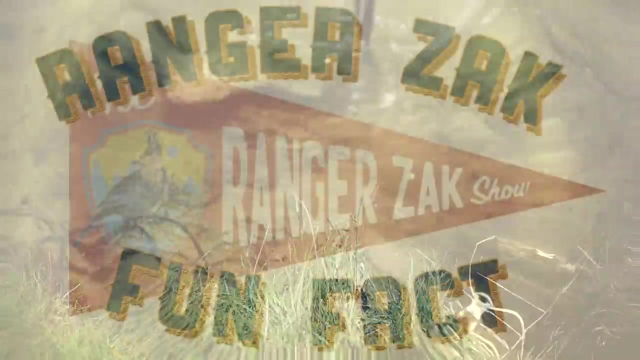 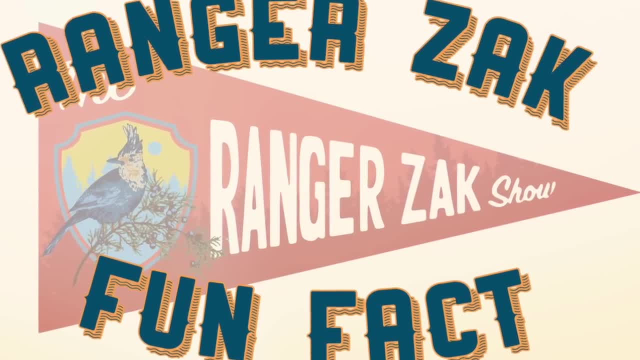 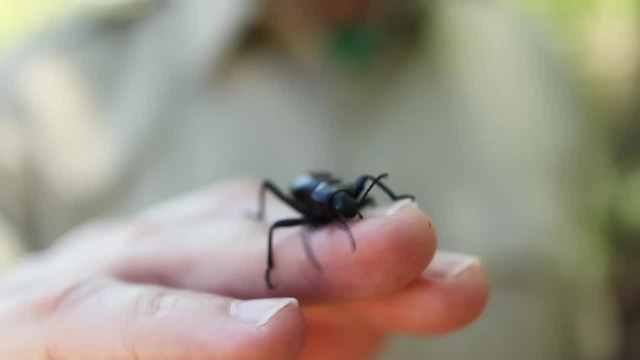 Adaptations, Adaptations, Adaptations, Adaptations, Adaptations, Adaptations. Are you ready for your Ranger's Act? fun fact, Yeah, Here it is. This is a stink bug and it's well known for being able to make a stinky. 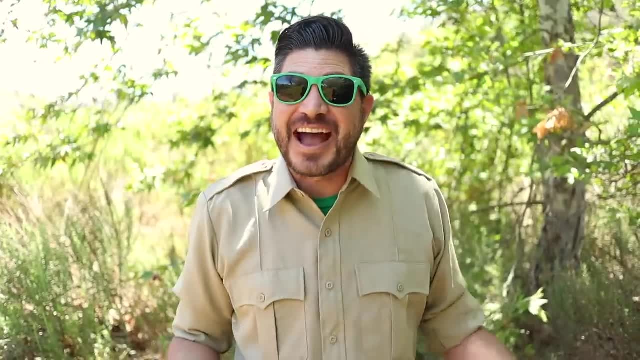 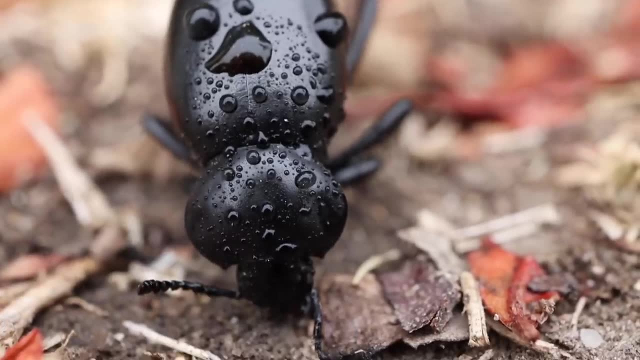 smell just like a skunk, But it also has a clever adaptation for gathering water. It'll stand on its head and collect dew on its back, which then drips down to its mouth giving them color. I hope it won't end up all over the world looking dirty inromantic as well. 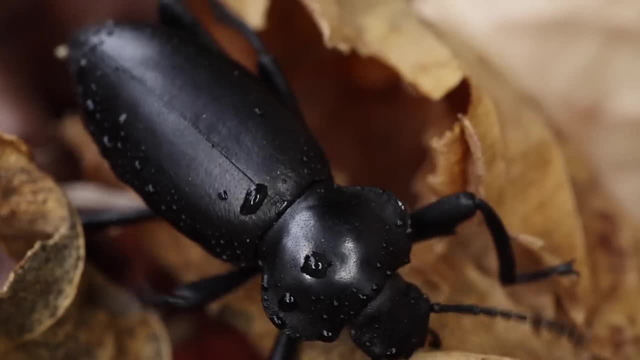 This was the most disgusting organ of the desert that I've ever seen. This is one of the best spin何. This is the one I've ever l센 about my own life. It's made of hay, archerg Et 뒤 It uses LIGHTS. 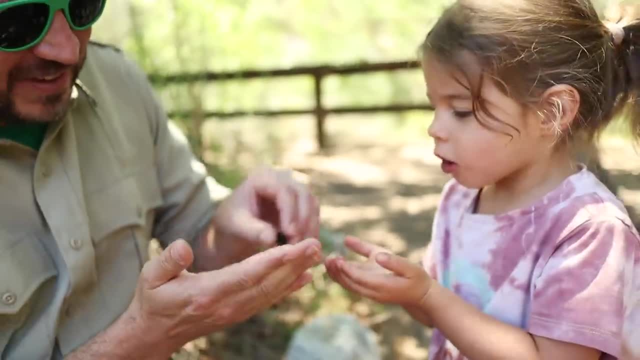 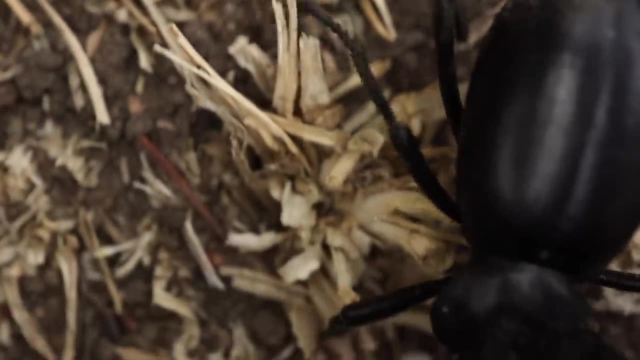 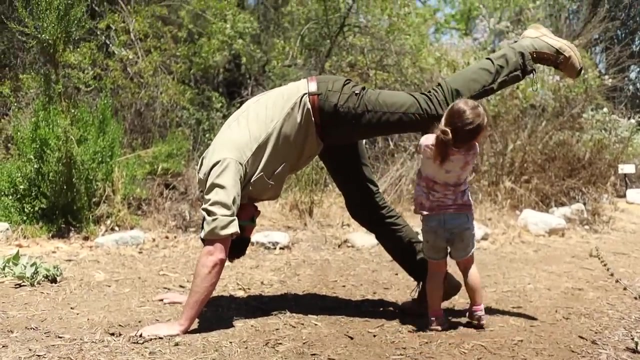 It uses gems, It uses TVs, It uses machines. It's nice to be able to see some. So not Sal, Entonces, Look that It's a tam hardesty Cro Wals, Really, Yes, It's difficult to cut it out. It's like you're create other animals. 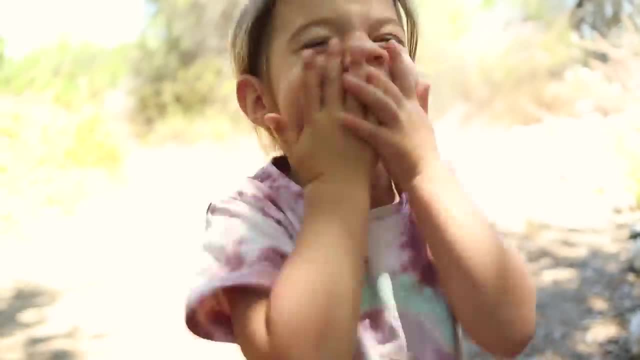 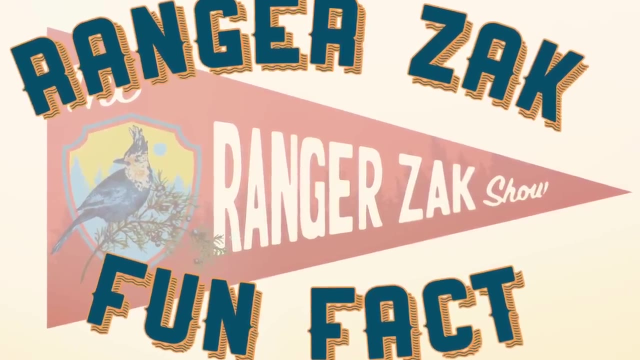 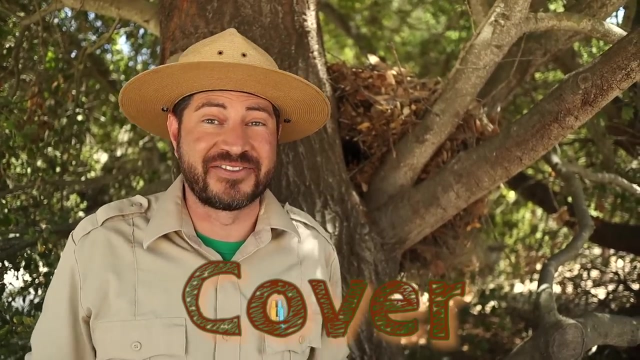 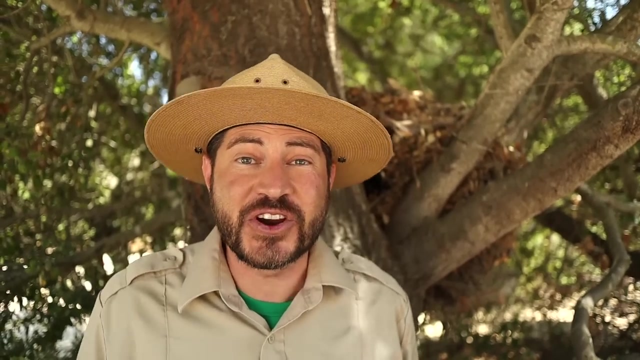 Taking books, You can see them all. anything but s? l師. Now, the third thing that a habitat needs to make a good home is cover. Cover can be made out of living things like trees and leaves and grass, or non-living things like dirt and rocks and cliffs. 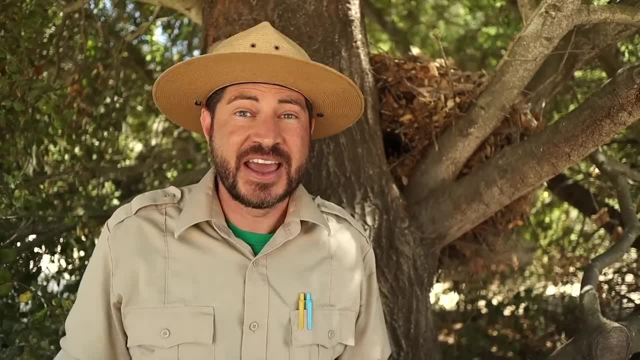 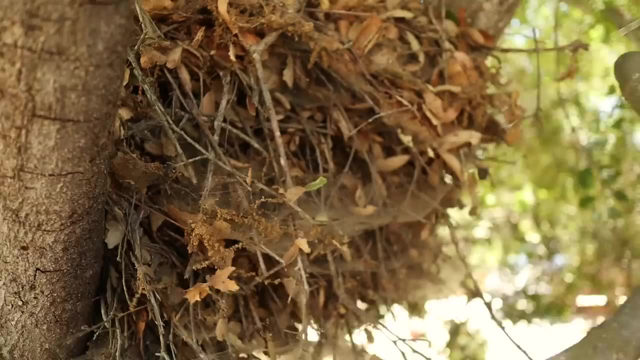 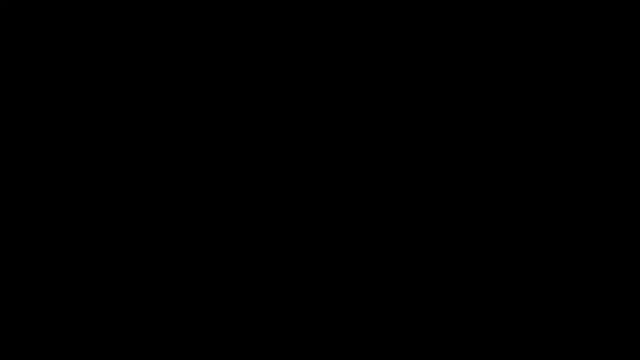 But no matter what it's made out of cover, all does the same thing: It provides the materials that animals need to make their homes. The wood rat behind me has used the cover in its habitat to build a nest. Let's see if anyone's home. 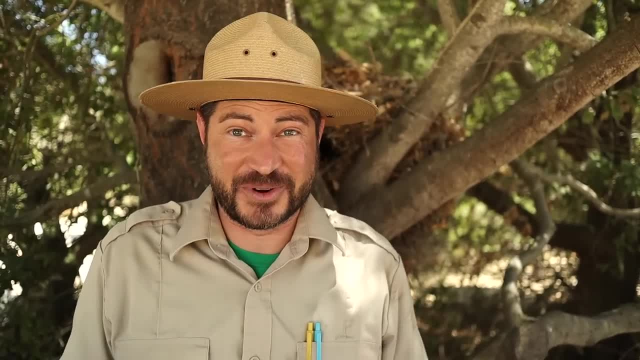 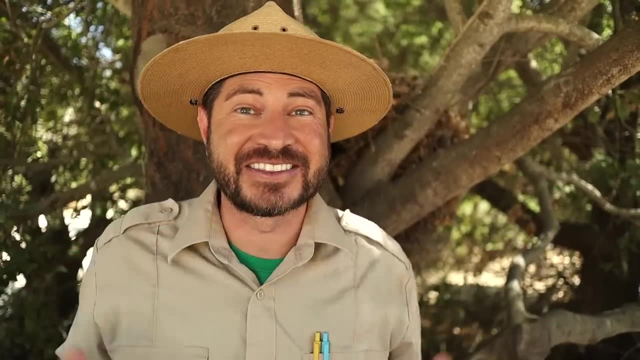 Cover also provides hiding places for herbivores to hide from carnivores, But carnivores can use cover to sneak up on their prey until they're ready to go In a palace. Let's have a look and see how other animals are using the cover in their habitat. 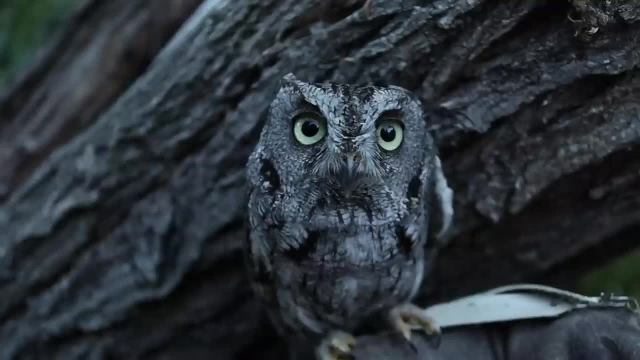 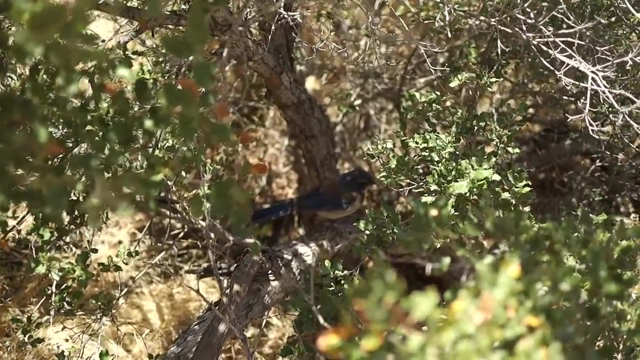 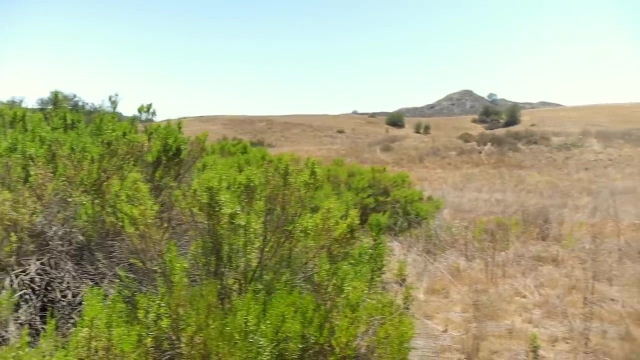 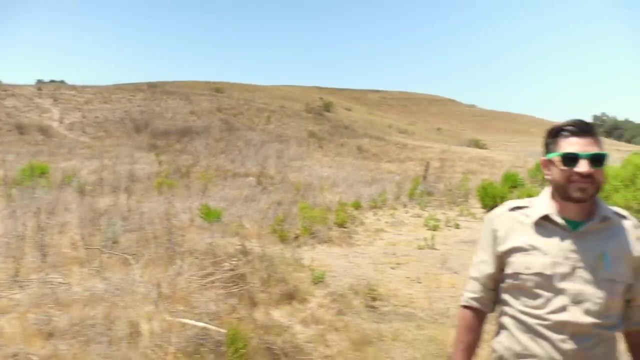 I'm going to try to hide it and see if anyone can see it. The last thing that we need to make a habitat a home is space Covering. one thing we need to do to make a habitat a home is that we need to have space. 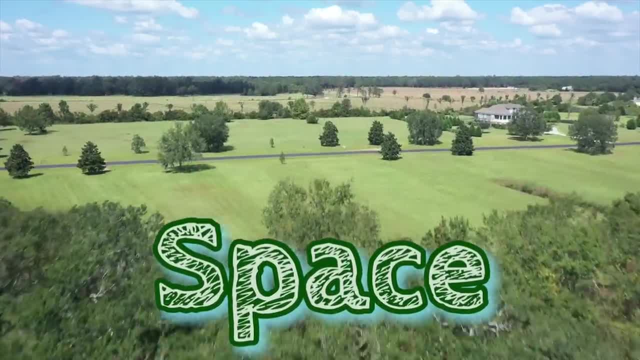 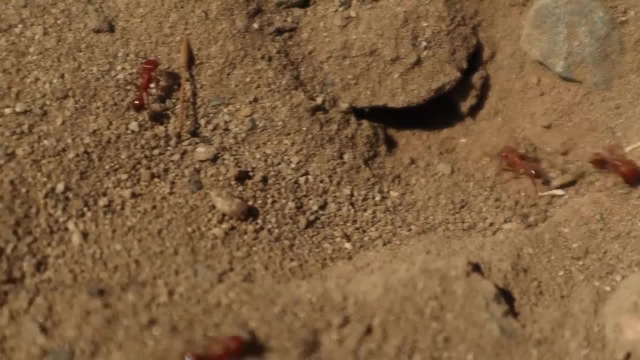 I think we need to have space for a lot of things. Space means that the habitat is large enough for a plant or animal to survive. Think of an insect. they may only need a tiny place to live to find all that they need to survive. Compare that to a bear or a mountain lion. and they need a lot more space to hunt, find a mate and raise their babies. Look at all this space. Here's a picture of a bear and a mountain lion. Look at this. Look at this. 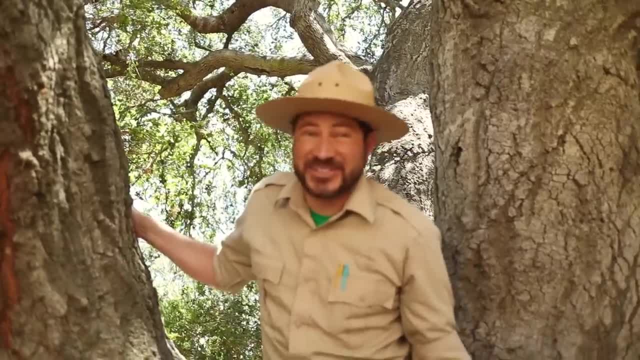 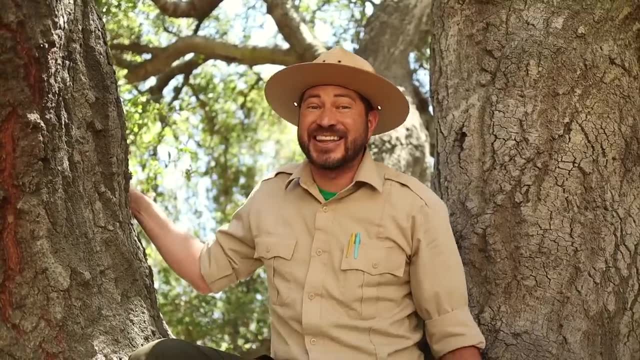 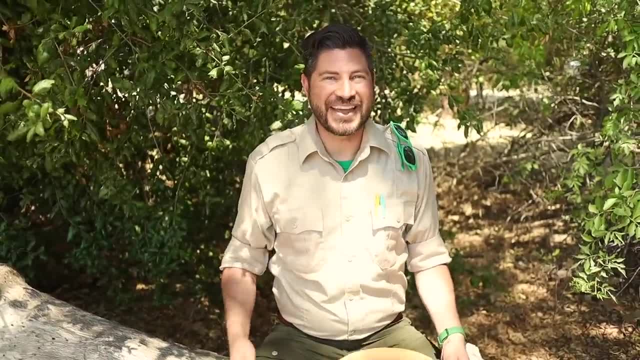 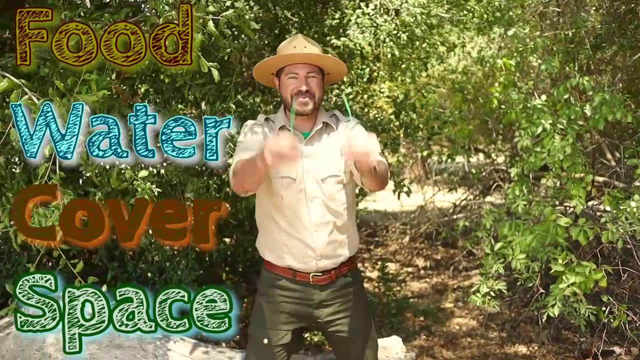 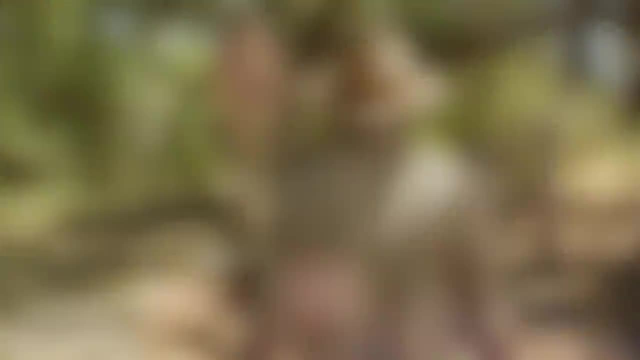 Today we learned that for a habitat to be a home, it needs food, water, cover and space. Let's head back to my habitat and wrap things up. Hi Junior Rangers. Welcome back to my habitat, the Ranger Station. Now, before we say goodbye, let's welcome back your friend and mine, Pearl the Squirrel. 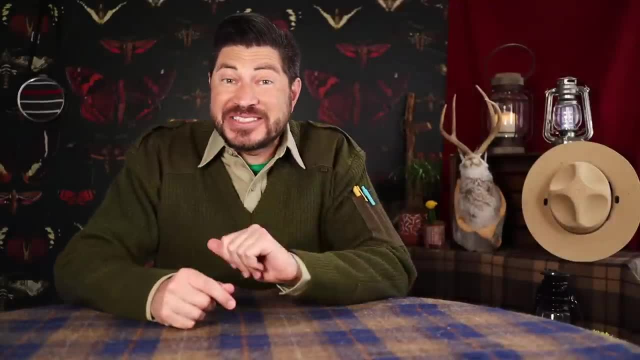 Hi Pearl, do you want to do the ranger roundup with me? Well, okay, let's do it. Hey Pearl, you want to do the ranger roundup with me? Well, okay, let's do it. Okay, let's do it. 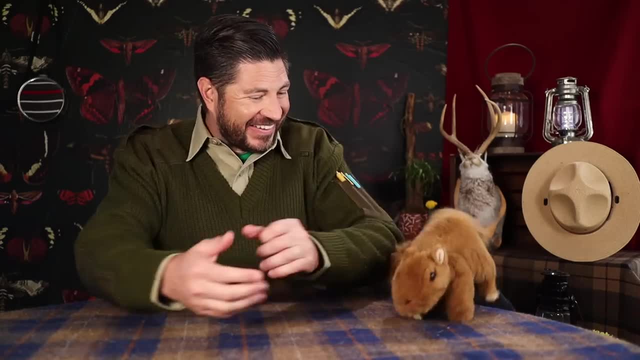 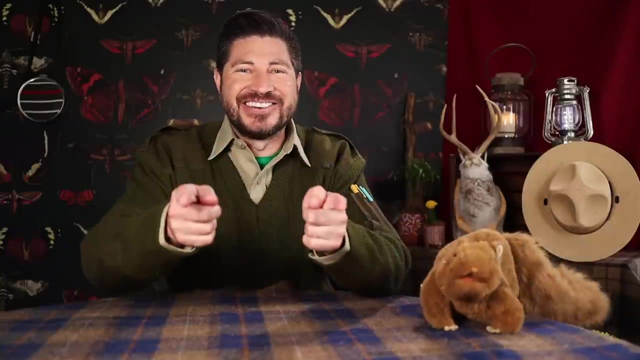 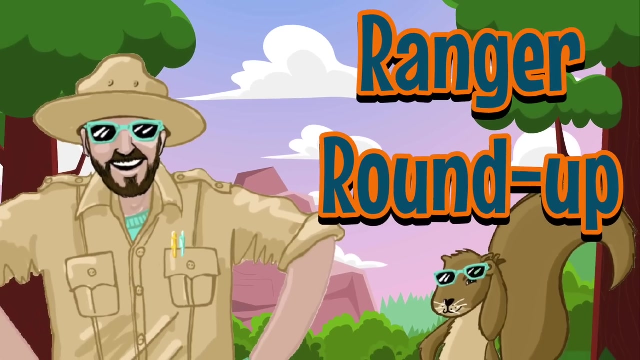 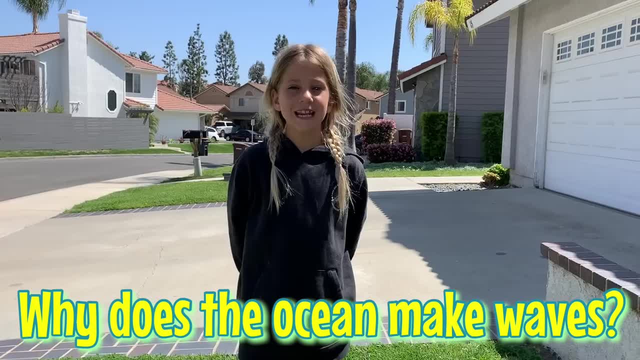 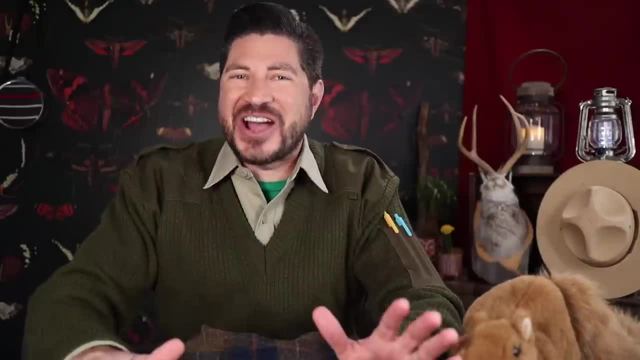 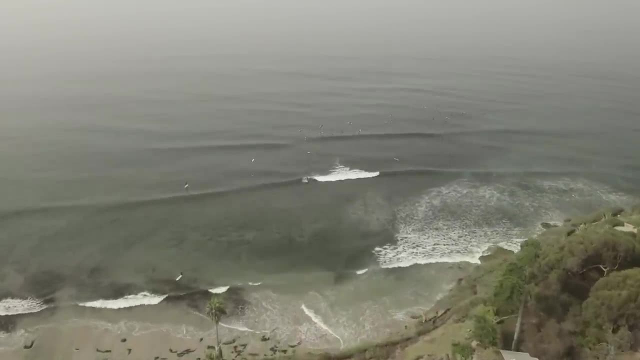 Hi, Ranger, Zach, I have a question for you. Why does the ocean make waves? Well, Liv, that is a very righteous question, But it's actually not oceans that make waves, it's wind. That's right. waves are created when wind blows across the surface of the ocean, creating 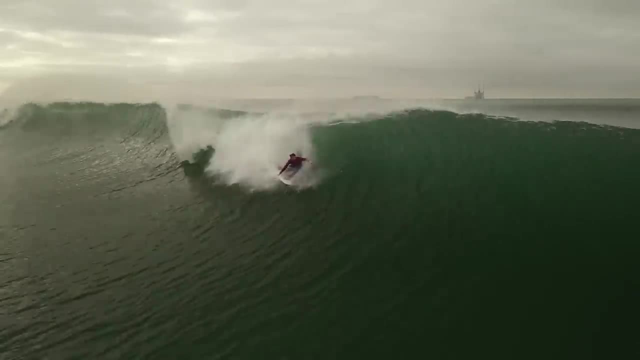 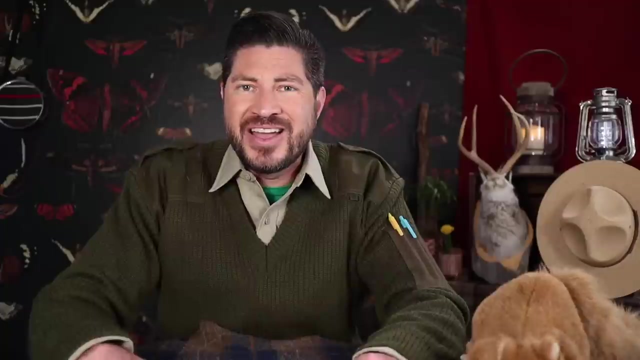 energy. When that energy hits a shallow coastline, it creates a wave and begins to break. This makes a killer tube that we can hang ten in brah. Well, I hope that answers your question. Now let's do the Junior Ranger Challenge. 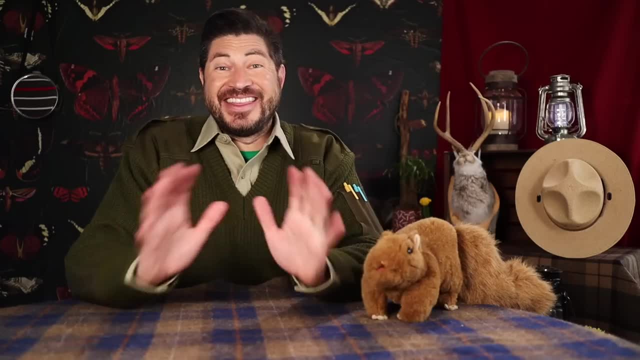 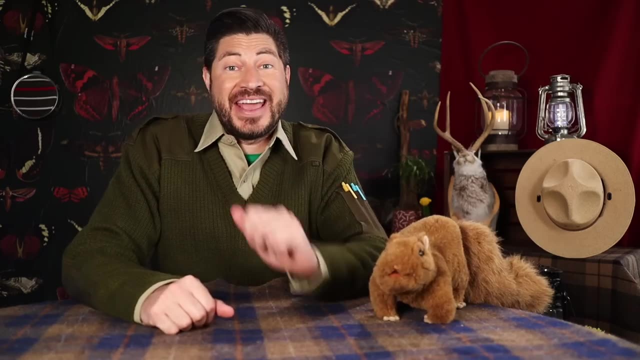 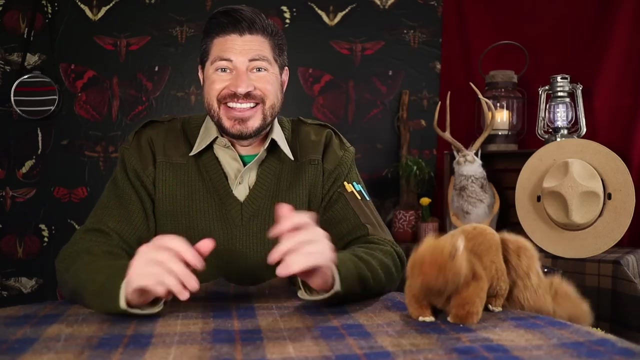 This week's Junior Ranger Challenge is to find a habitat near your home and find one plant and one animal that makes its home there. Take a picture of the habitat and share it with me at the rangerzachshow on Instagram And you can be featured as one of our Junior Rangers of the Week. 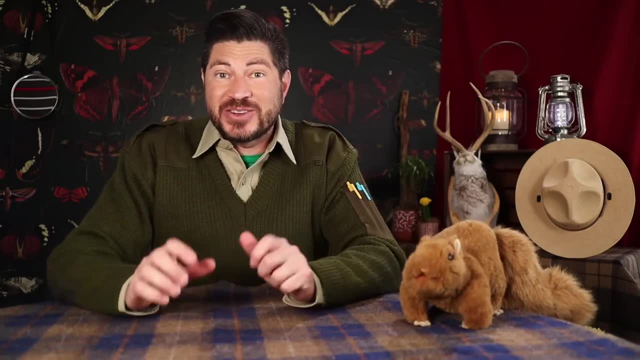 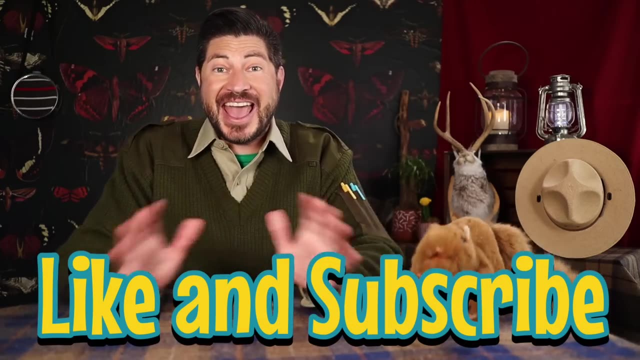 And don't you forget Junior Rangers. new episodes of the Ranger Zach Show come out every Monday And make sure to like and subscribe. See you next week. And don't forget to subscribe to our channel so you don't miss any of our exciting adventures. 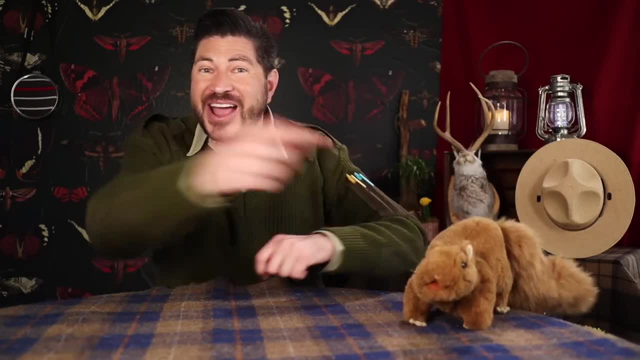 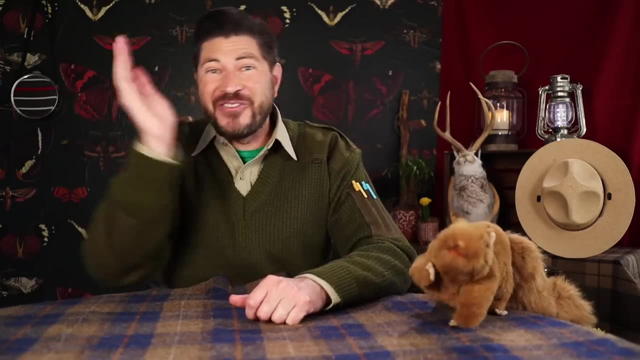 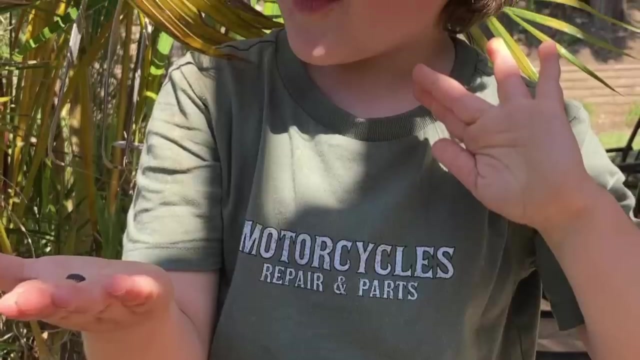 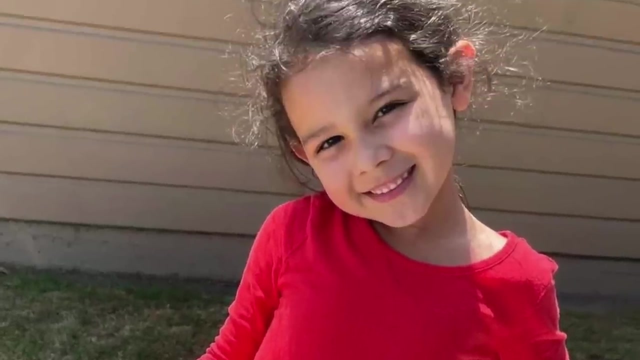 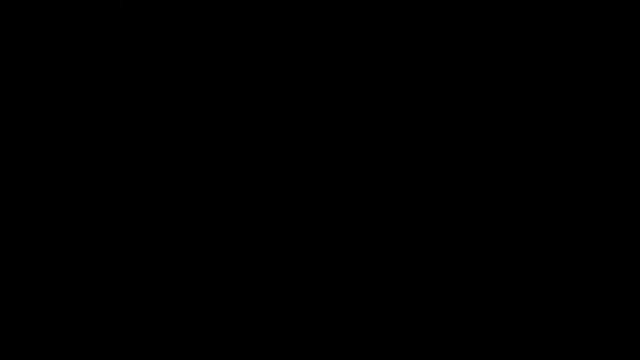 So until next time, Junior Rangers, there's a world of adventure right outside your door, So get out there and go explore. This is Ranger Zach and Pearl. the Squirrel over and out.